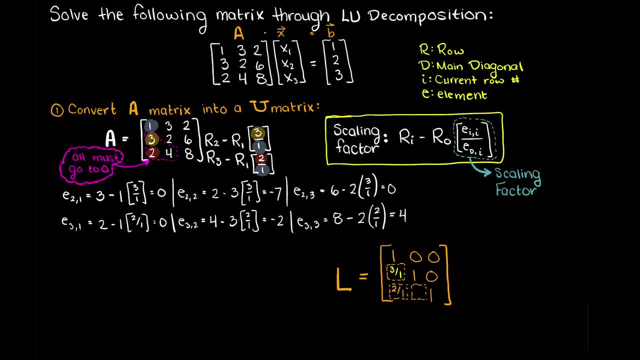 scaling factors we have been finding Alright. so, as you can see, we now have our first column just how we want it. Now let's repeat the same process for our second column. As you can see, there is only one row that we need to conduct row operations on. 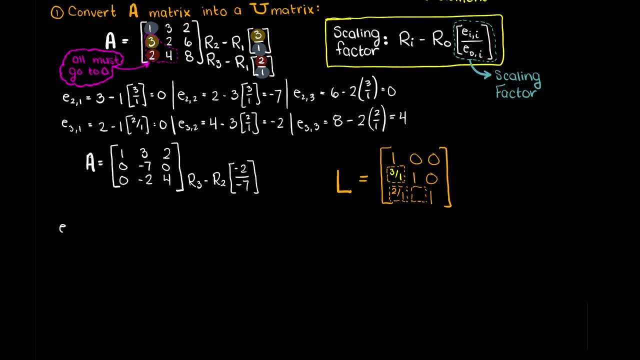 Therefore, we have row 3 minus row 2 times our scaling factor of minus 2 over minus 7.. And again, just go ahead. We can also add the scaling factor as our final missing piece of our L matrix. Now that our U and L matrices are solved, we can use the following formula to solve for: 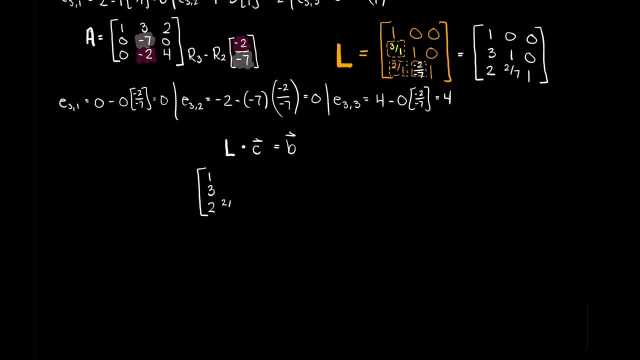 our constant vector values which, as we learned in the LU decomposition theory video, we can use to solve for our A matrix. So, as you can see here, Once we write out all of our matrices, the only thing we need to do is complete a quick 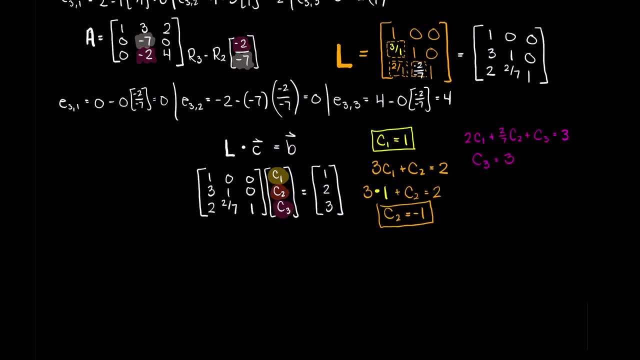 forward substitution to find all of our missing constant values. After solving, you can see that C1 is equal to 1,, C2 is equal to minus 1, and, lastly, C3 is equal to roughly 1.2857 after truncating our fraction for simplicity. 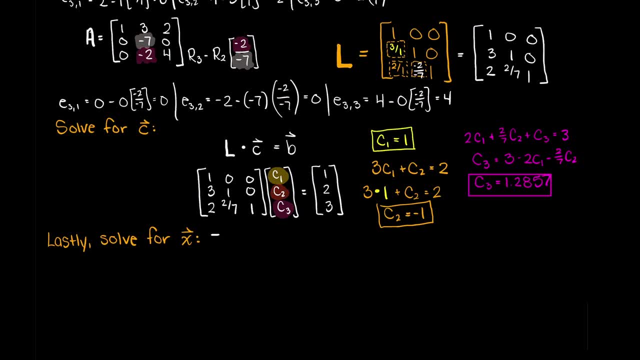 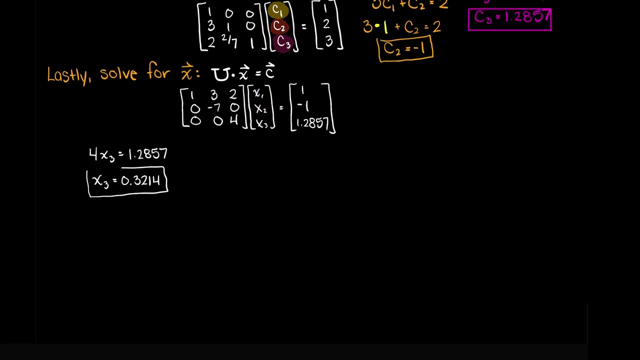 Our final step in completing our LU decomposition example is solving for our unknown x variables. As you can see here, this is done by using backwards substitution, Which is what we want, Which I will go ahead and complete for you right now. There we go. 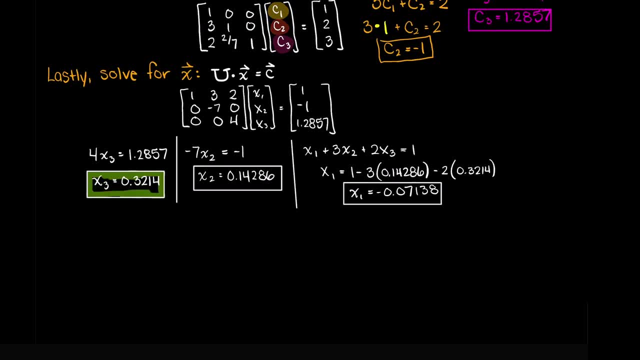 We have: x3 is equal to 0.3214,, x2 is equal to 0.14286, and x1 is equal to minus 0.07138.. Ok, If you wish to validate your answers at this point, you can plug these variables into your. 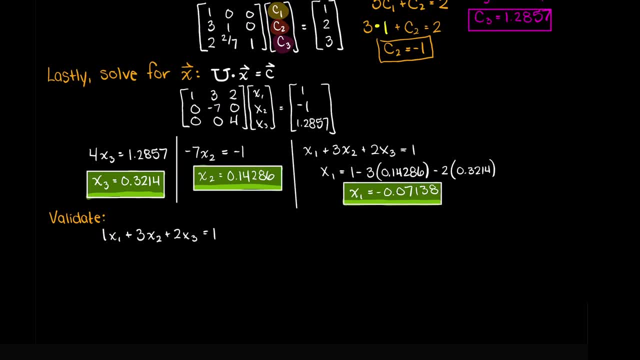 A matrix that we had earlier and this should solve your system of equations. And it does indeed solve our system of equations as expected. Therefore, our solution is correct. I hope that this video helped your understanding of how to solve a matrix. If you enjoyed, please like, subscribe and consider checking out our YouTube memberships.